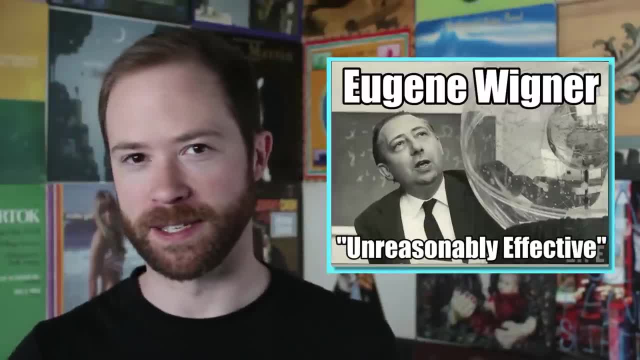 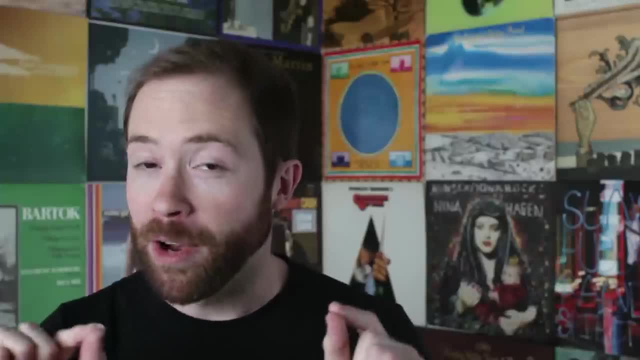 unreasonably effective when put to use in all other sciences. But in light of its beauty and effectiveness and in spite of its importance, there is a thing you can argue about it. You can argue where it comes from, where biology is the study of living organisms. physics- 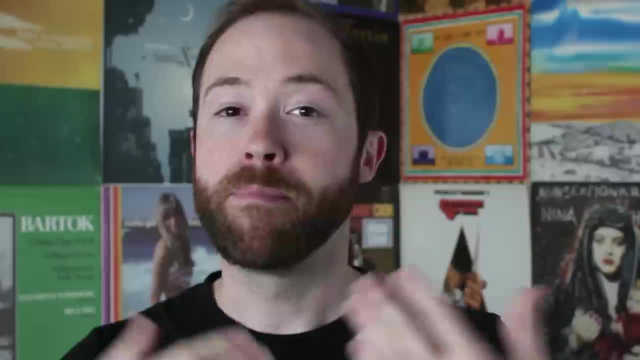 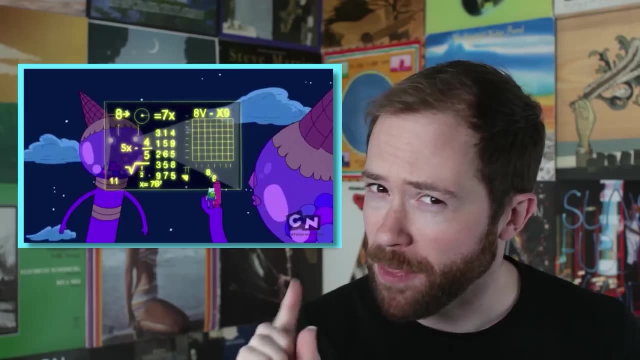 the study of the universe and its forces. chemistry the study of chemicals. math is the study of math. Unlike all the other sciences, math lacks an empirical component. You can't trust me on this one. see math happening Like sure if you have one Wheezy Waiter. 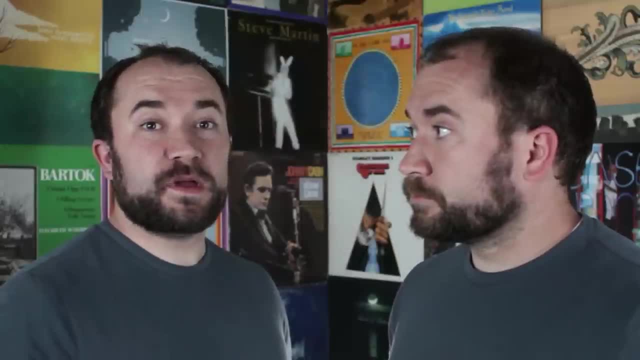 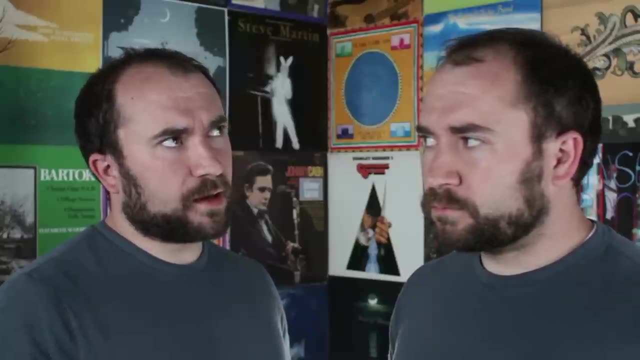 and you add one Wheezy Waiter- clone, You have two Wheezy Waiters. But is this oneness a part of me? Is this two-ness a part of both of us? I like to think that I'm a part of you. 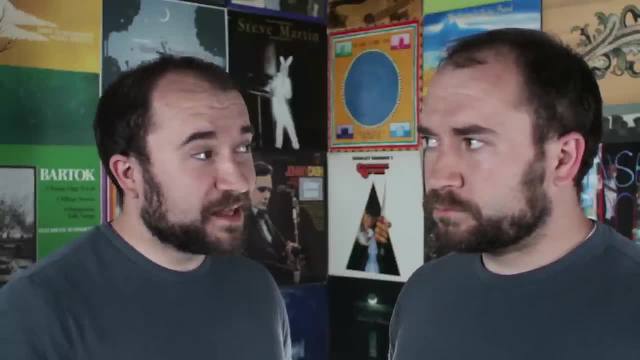 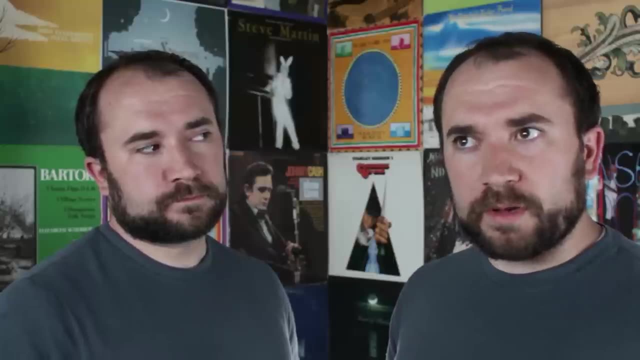 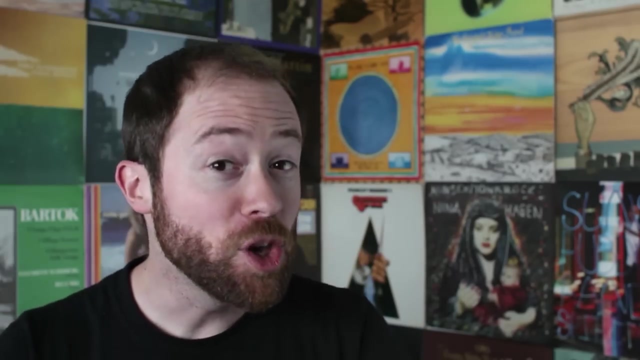 I mean, sometimes we even finish each other's. As I was saying, are these ideas, features of the universe and the stuff in it, Ideas like one, two parabolas, calculus, subtraction, double subtraction, Or are they a product of the human brain? 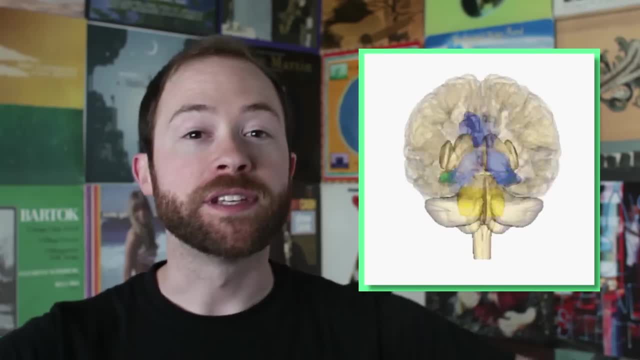 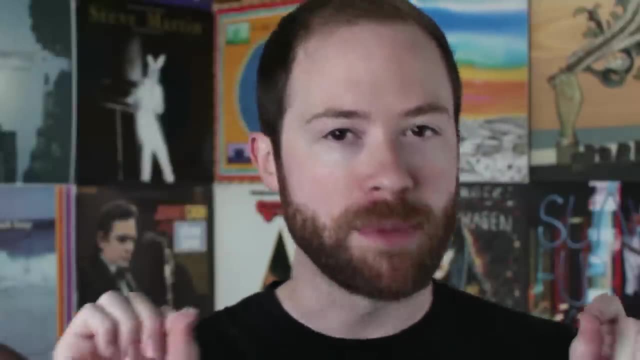 in all of its genius and splendor. In other words, do people discover math or do they create math? Saying that people discover math, meaning that it exists regardless of whether or not there are people, is the most popular position among the people. 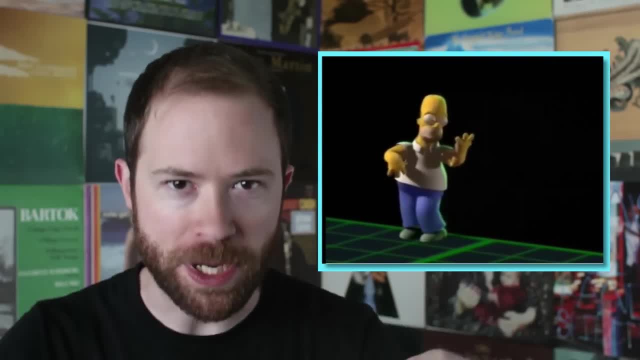 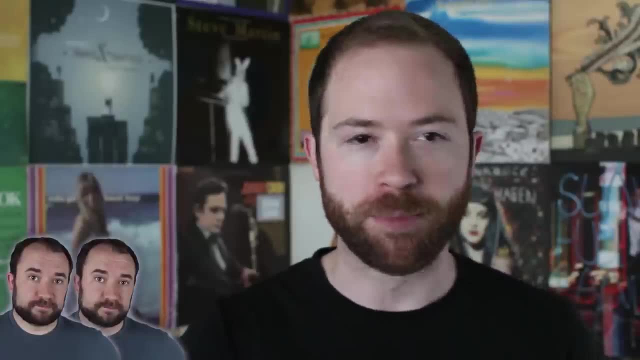 It's the most popular position amongst mathematicians. Mathematical realism says that math is real, that it has an objective existence. It's like stuff- And I don't mean objective- like two Wheezys plus another two Wheezys equals four Wheezys, regardless of your opinion. 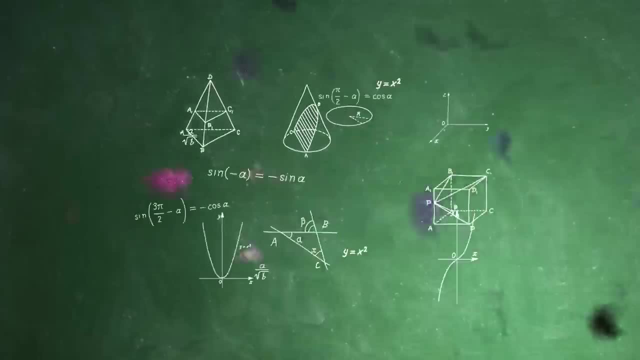 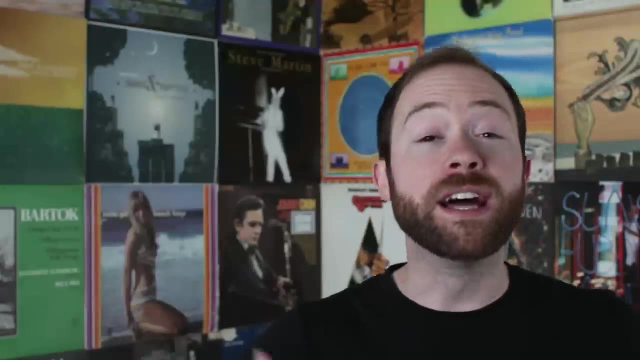 But objective. like mathematical concepts exist disembodied in the universe And, as humans with awesome brains, we uncover them and bring them into practical use. New mathematical concepts are like undiscovered species: We just need to find them and in doing so, 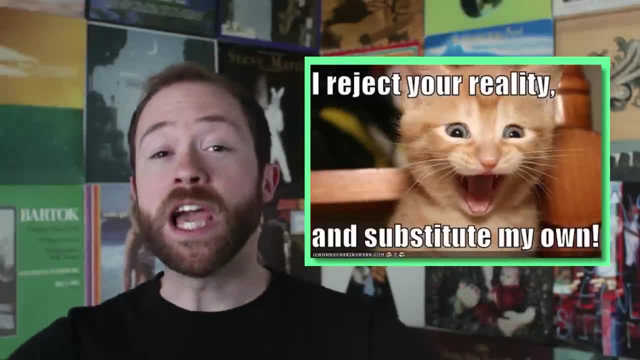 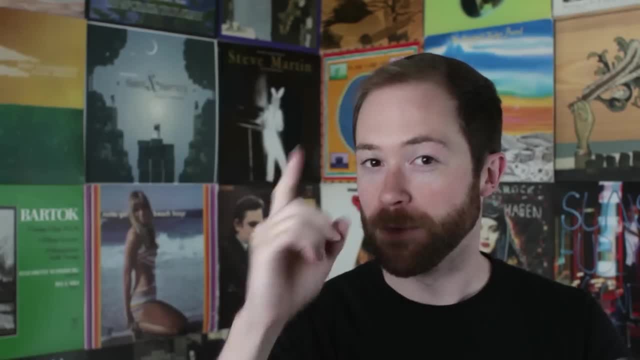 add to our set of mathematical knowledge. The anti-realists say that the only reason we have that set of mathematical knowledge is not because we discovered it, but because we created it. They say that math comes from the human brain and nowhere else, And there are a bunch of different variations. 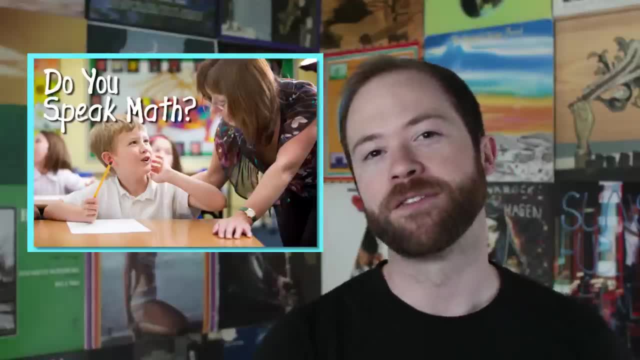 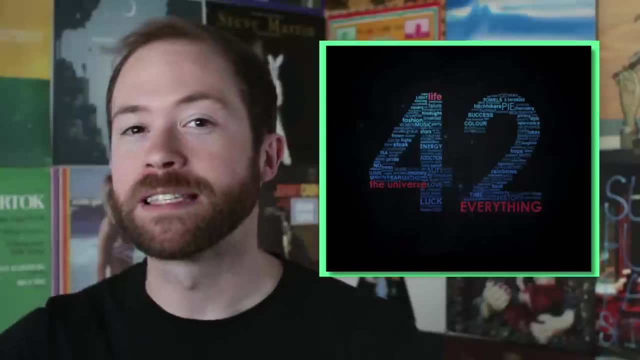 on this idea. like math is a metaphor, math is a language. My personal favorite is called fictionalism. Fictionalists say that square roots, the derivative of tan, x, 42, and all other mathematical concepts are part of a fiction. 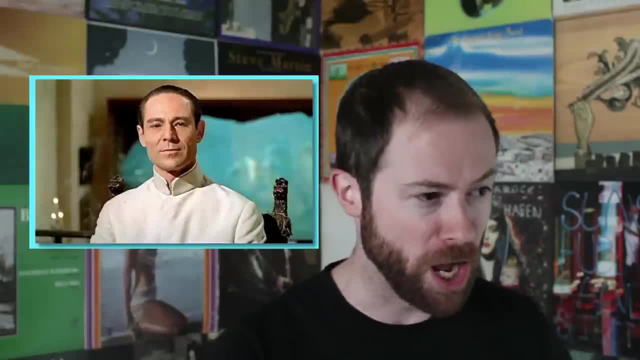 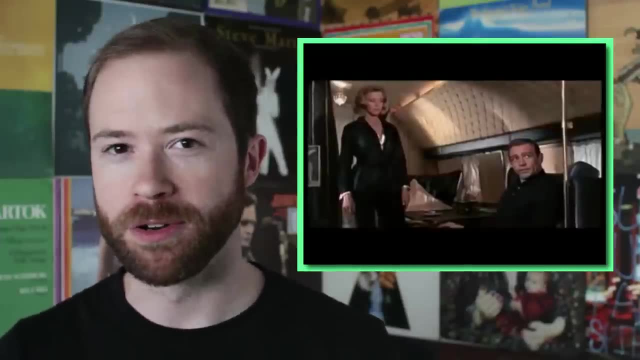 They are the elements of a story, the story of math, in the same way that Dr No and a car with missiles in it are elements of the story of James Bond. 10 divided by 2 equals 5 is about as true as James Bond ordered his martini: shaken, not stirred. 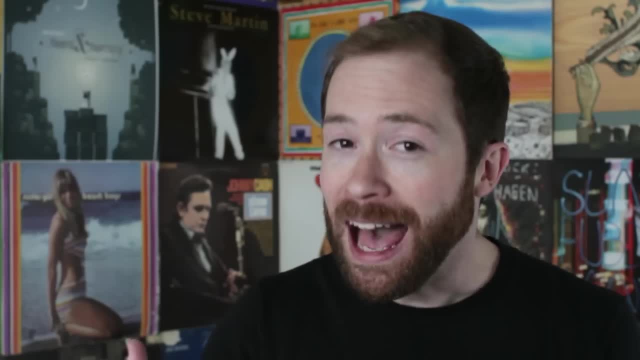 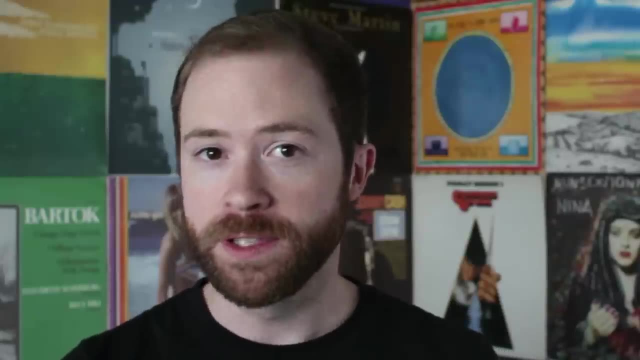 Within the construct of the story it makes perfect sense, But outside the story- 5,, 10,, James Bond and his martini don't actually real. What we do is we use the story of math, which is very good and very complete and totally mathematical. 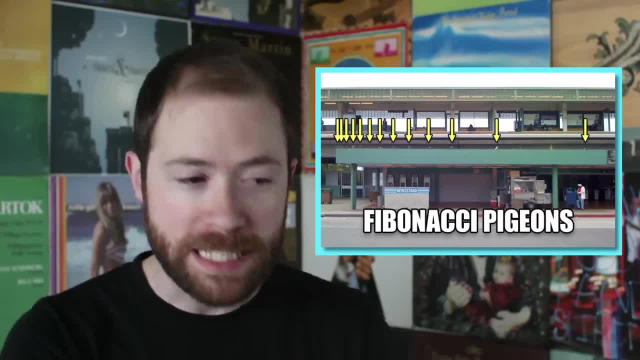 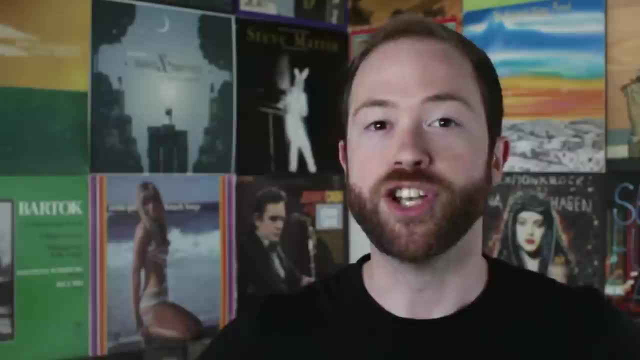 Good job us to describe real things which do not themselves contain or perform math Like. Does an unladen European swallow need all of this math in order to travel at 24 miles an hour? No, Of course not, And furthermore, your mother was a hamster. 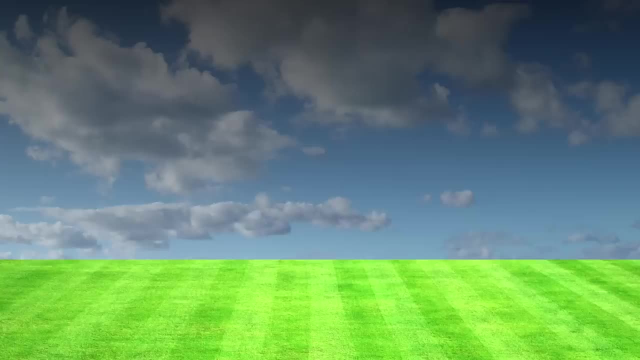 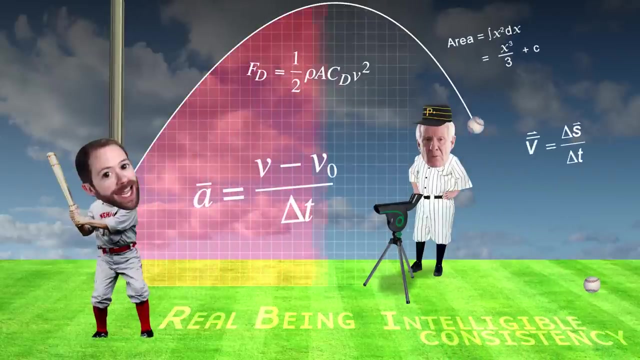 and your father smelled of elderberries. Philosopher Alain Badiou says that mathematics is thus a rigorous aesthetic: It tells us nothing of real being, but forges a fiction of intelligible consistency. Now, this is a nice, friendly, philosophical conversation. 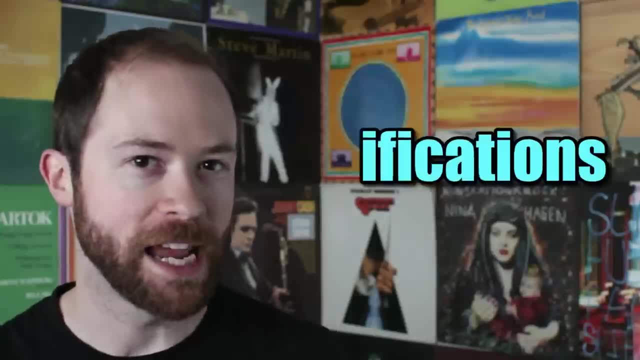 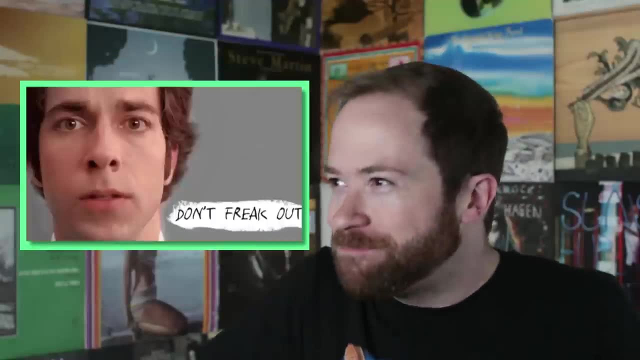 until we start to consider one of my favorite if-ications, ramifications Like what exactly is at stake when we're considering the source of mathematics. I mean, I don't want to alarm anybody, but literally everything. For mathematical realists, math is about truth. It is true that when you group 5 of something with another 5 of that something, you have 10 of that something. It is true, We can prove it. So if math and its operations don't exist, are we saying that truth or a version of it doesn't exist? 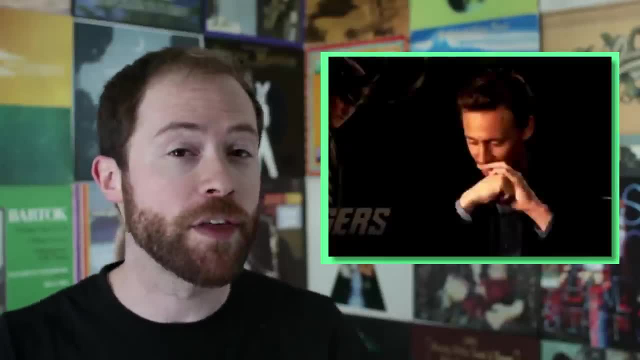 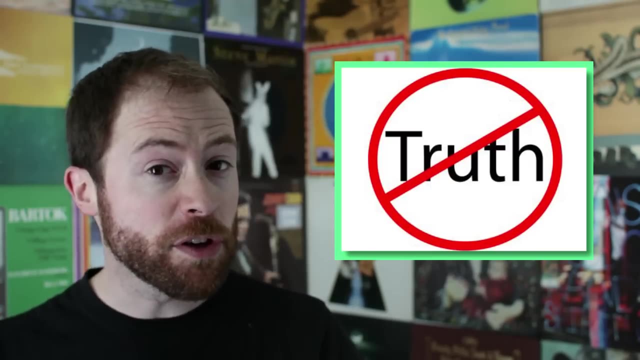 Some anti-realists would say that there is only 10 of that something, because we are there to count it and perceive it and that objective. There is no group, no 10, and no mathematical truth, Or maybe it's just math that's at stake. 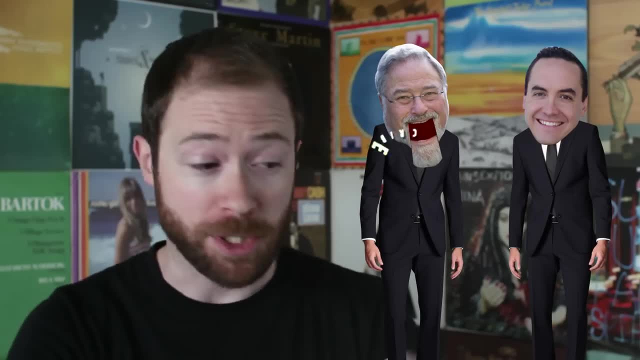 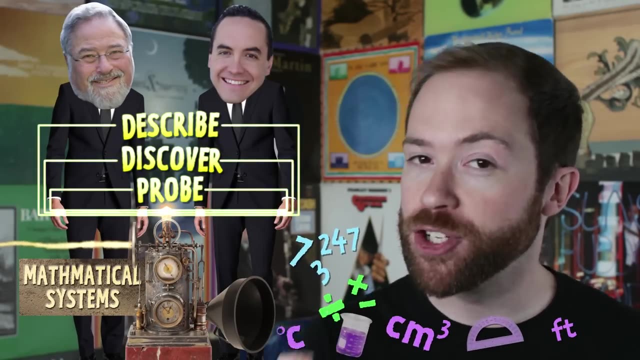 Cognitive linguists. Lakoff and Nunez say that humans, because we want to describe, discover and probe, are great at inventing systems that help us do that: numbers, operations, even measurements. Lakoff and Nunez say that math is. 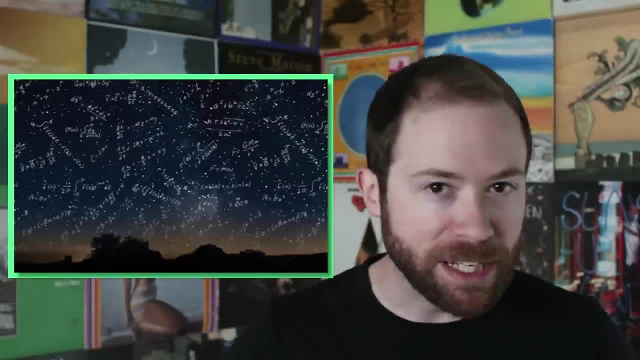 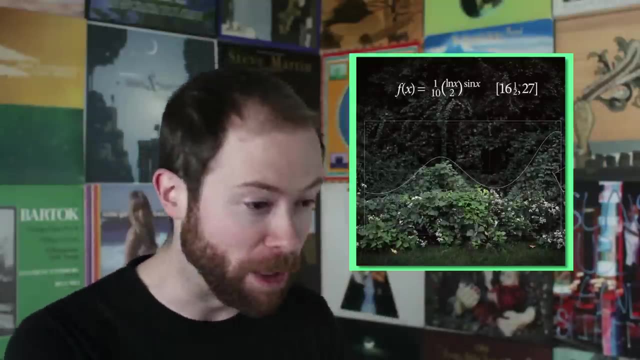 able to model regularities in the universe which are not inherently mathematic, but are modeled and understood through math by humans. If there existed something better than math at explaining and modeling the world, then we'd use that instead. Sources for all this in the doobly-doo, a word I invented. 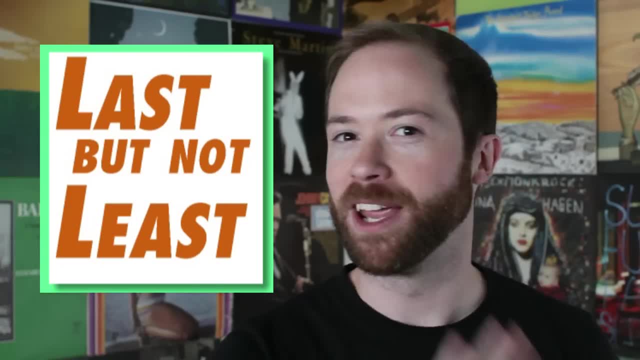 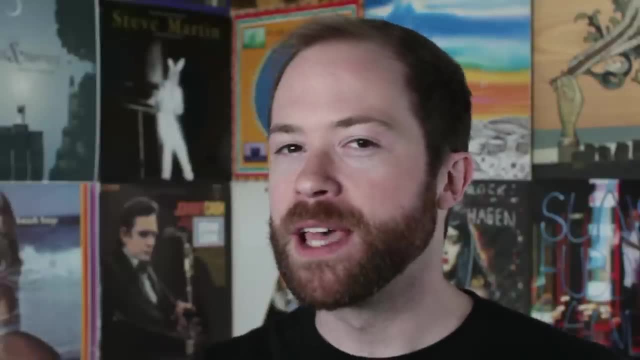 Which brings us to the last and, I think, most important point in this very weird conversation, Seeing as how math is only provable with more math, a tautology arises: The only math which is known by humans is the math which is knowable by humans. 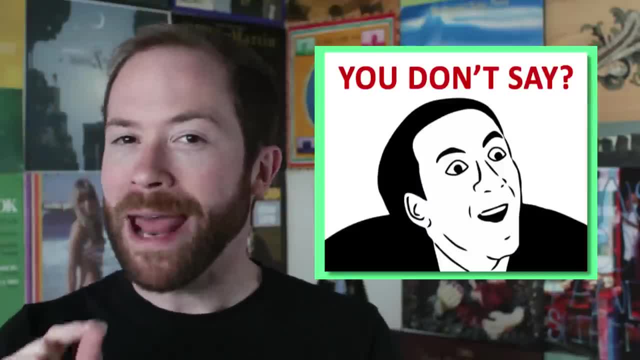 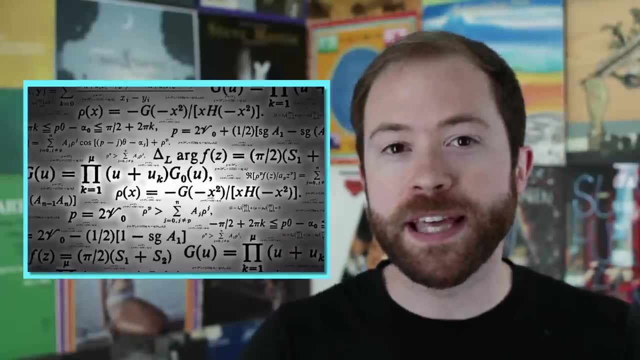 It might seem obvious, but it's really important, because mathematical realists believe that, beyond the math we currently know, there is more math. We believe in an objective mathematical universe that contains concepts we might one day discover. we might never discover, and for whatever reason. 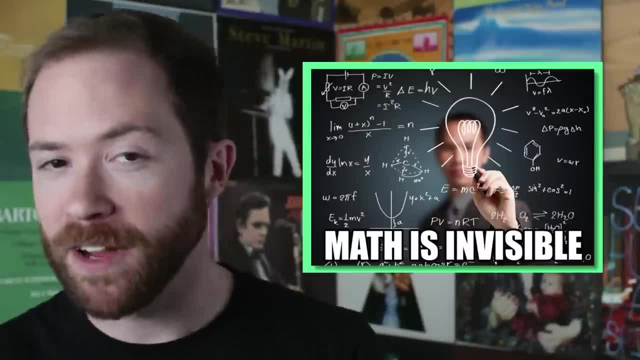 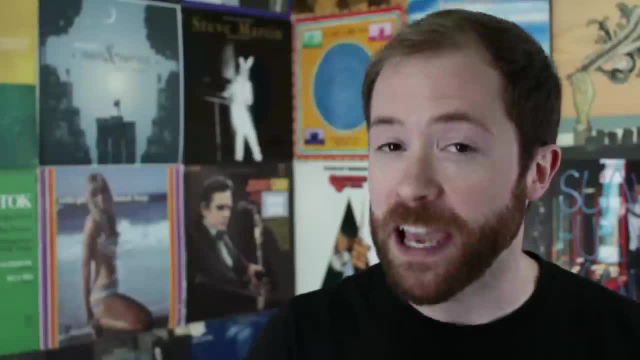 might never be able to discover, And in the absence of a direct observation of mathematics, in the same way that a biologist can directly observe cells. mathematical realism boils down to a kind of faith, a faith in a mathematical entity or set of entities which is out there in the universe. 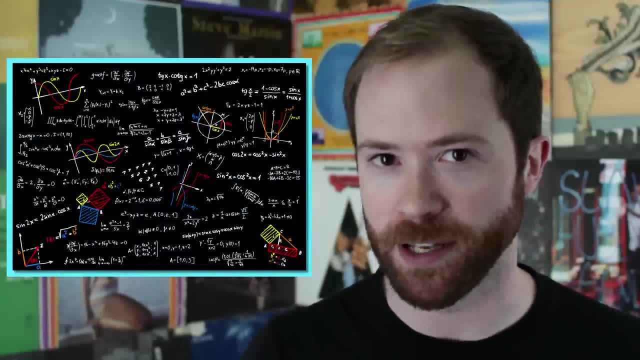 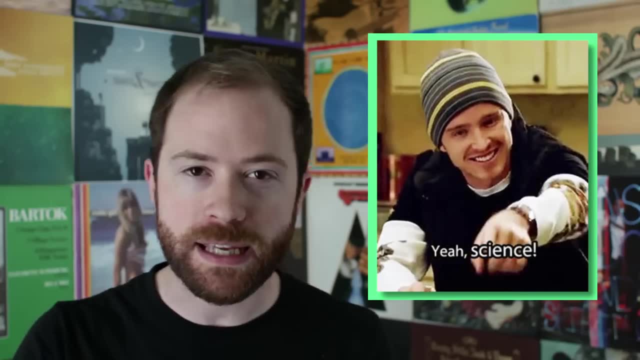 waiting to be discovered and would be there regardless of if they're humans or not. Now, to my ears, the belief in an external mathematical universe to perceive or directly interact with sounds a lot less like science and a lot more like the opposite of science. 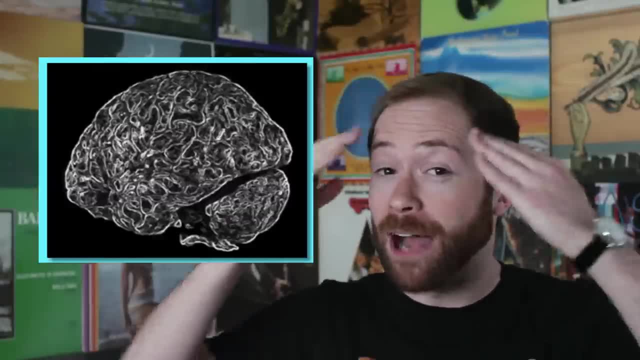 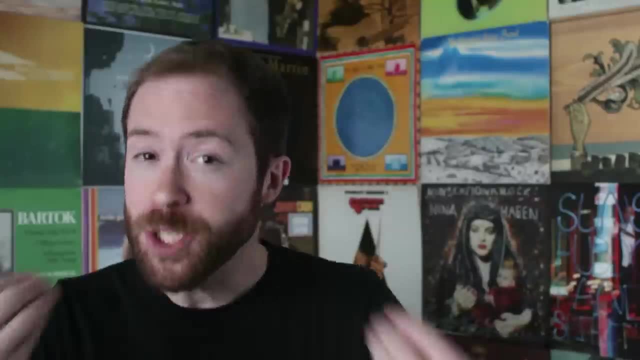 So does this mean that I think realism and the idea that mathematics exists outside of the human brain is false? I really don't know. Personally, I think anti-realism is more interesting. But if I really knew it was true, I would probably have a Nobel Prize in physics. 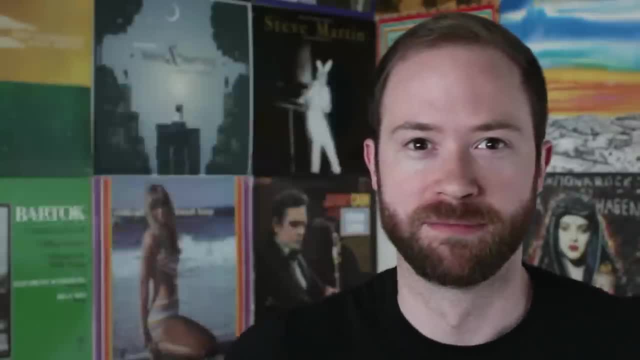 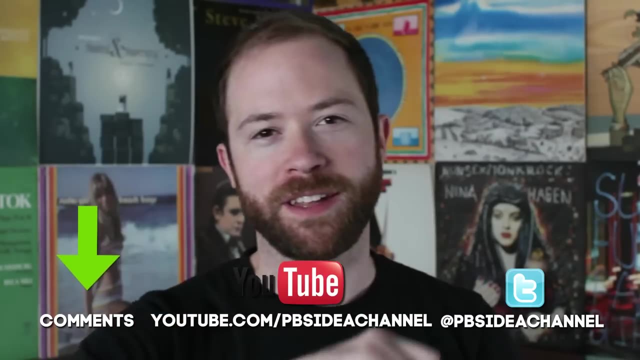 or be Brahma, the creator of the entire universe. What do you guys think? Does math exist in the universe, or does it come from the human brain? Let us know In the comments, And if you're not too offended, that I called your mother. 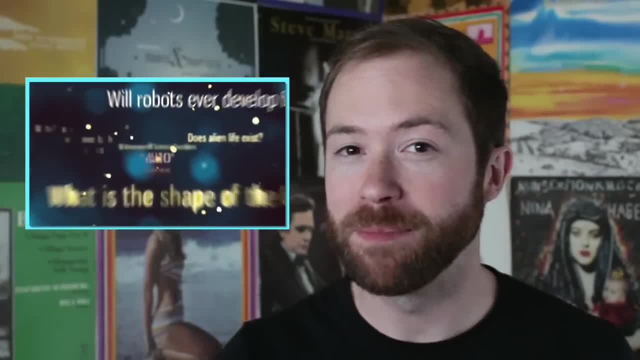 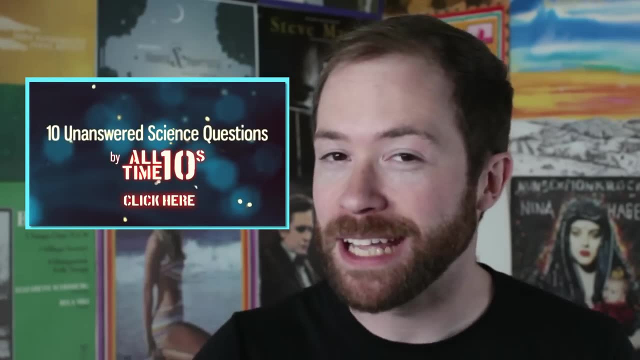 a hamster. please subscribe. This video is also part of an amazing all-time top 10 super collab, So we'll put an annotation somewhere here And you can see all of the other videos that people made about unanswered science questions. It's all crazy, interesting and mind-blowing. 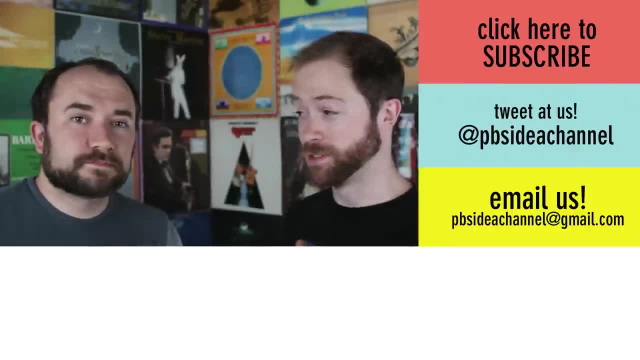 You should watch every single one of them twice. First of all, an extra big thanks to WheezyWaiter for coming by Idea Channel And if you aren't watching Craig's new channel, The Good Stuff you've got to get on that. 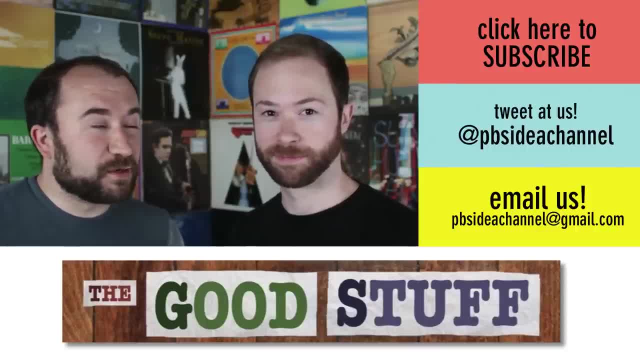 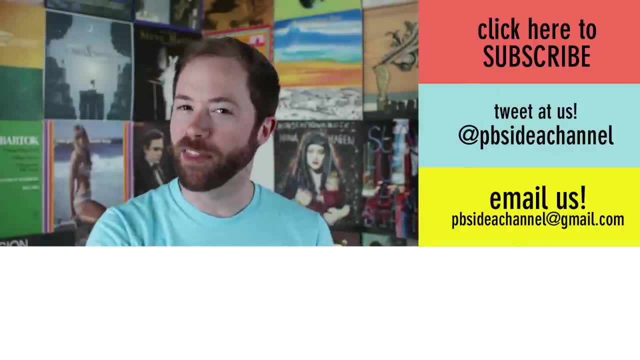 It's pretty good Stuff, Mm. Yeah, we make that joke a lot. OK, three additional news items. One: yes, I am wearing a different colored shirt. Please write a comment about it. Two: in our online-offline video. 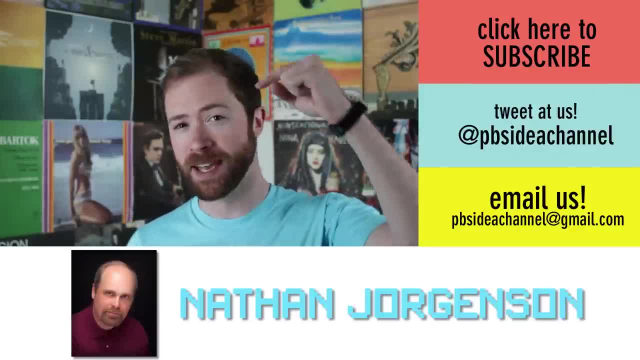 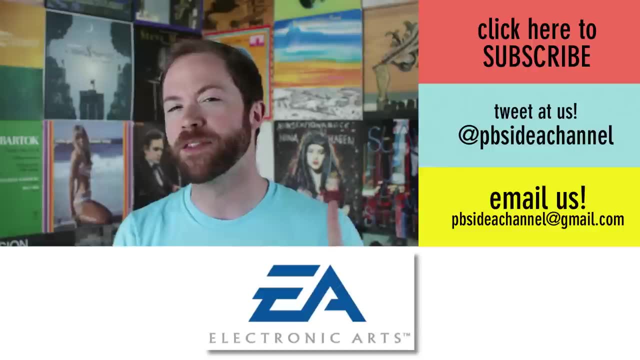 we didn't talk about the work of Nathan Juergensen, who we should have, So we'll put some links to his stuff in the description. Three: EA has released a statement saying that their relationship with arms manufacturers is a little more complicated than the media. 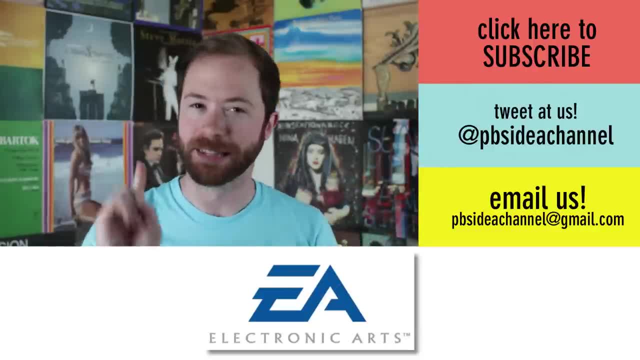 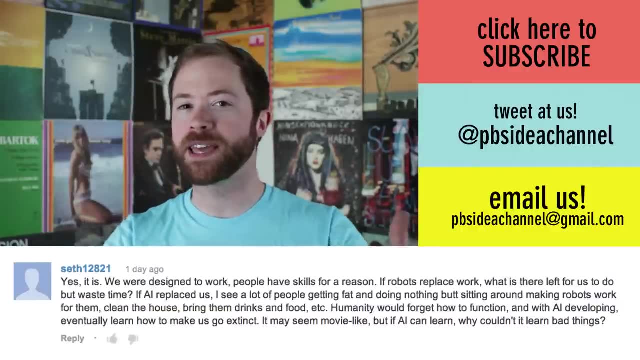 has made it out to be. So also some links to that in the description. Now let's see what you guys had to say about the ethics of developing AI. Seth12821 says that developing artificial intelligence might be unethical because he imagines a kind of WALL-E-ish universe where all of the humans 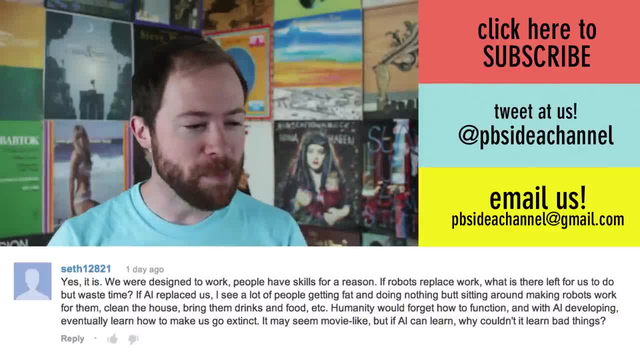 are fat and lazy because the robots are doing all of the work for them. I don't know. I think it's maybe part of human nature to always want to do stuff, But we'll, I guess we'll see how it turns out. 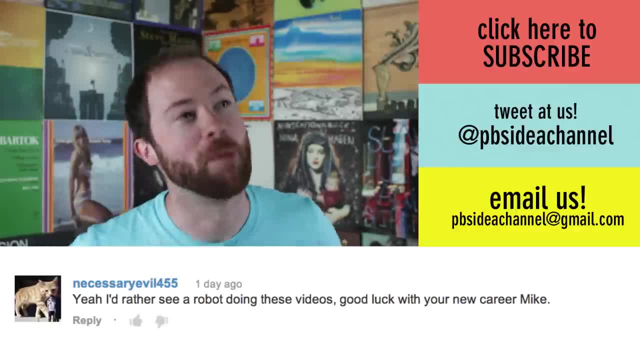 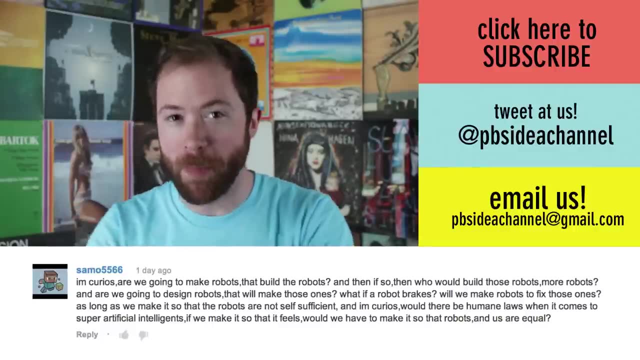 Well, NecessaryEvil455,, I'd rather see a robot writing comments. Hm, Actually, spam is kind of irritating. Sammo5566 wonders about the slippery slope of robots that build robots and then robots that build robots, that build robots, which, yeah? 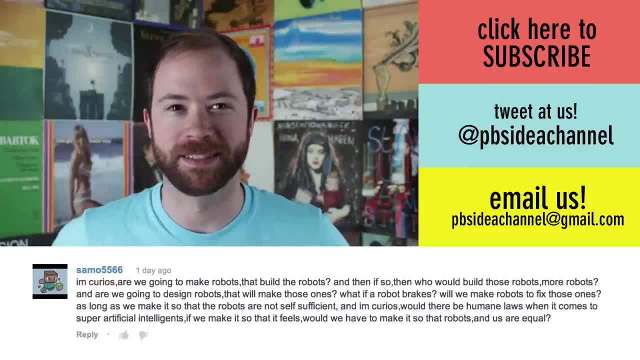 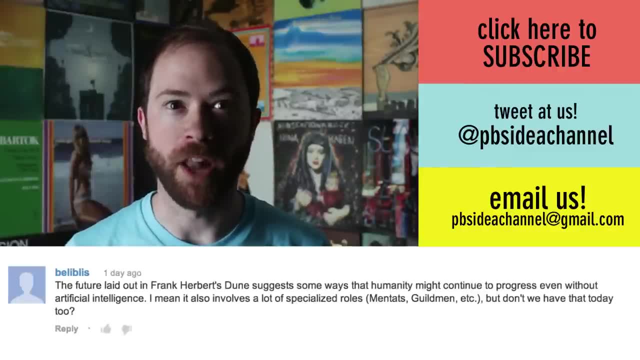 and then it's robots all the way down. I don't know. Let's just, let's hope that they're nice. Insert term. Insert theme. There is no fear. Fear is the mind killer. The spice must flow: BagofGroceries and ShyGuyXXL talk. 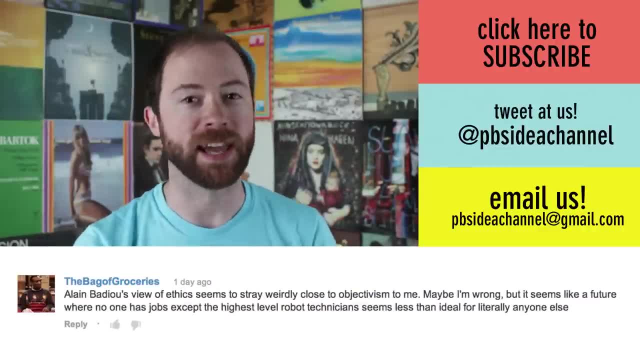 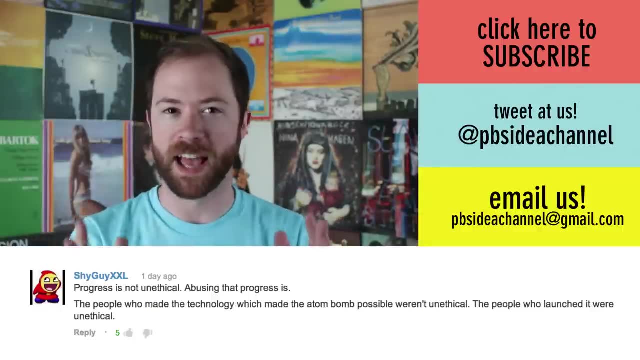 about how an objective idea of progress can be a dangerous thing, And I totally agree, And actually so does Alain Badiou. We didn't have time to talk about it, but he talks about how, if you let progress take on a totality like if it's the only thing that you're. 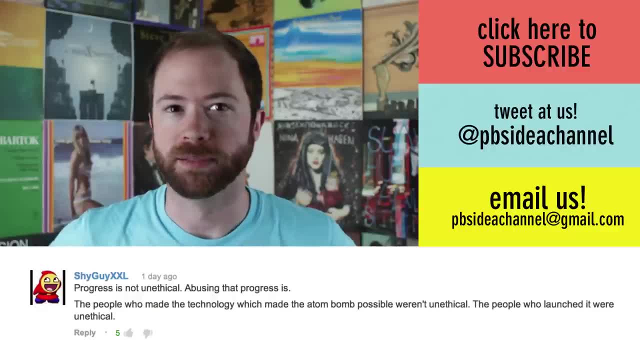 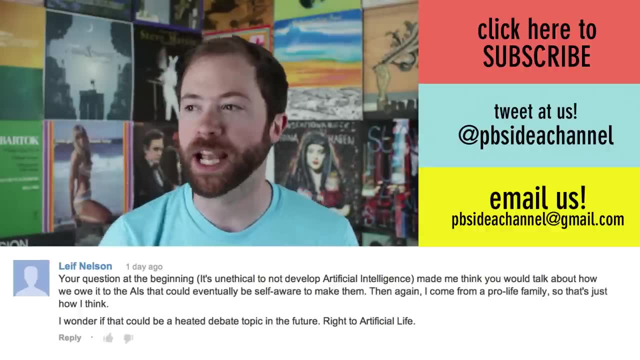 focused on, you're going to get yourself in some deep water, some future trouble. LeafNelson and a couple other people touch on the other ethical question related to AI, which is: Is it ethical to create a consciousness and then somehow regulate that consciousness? 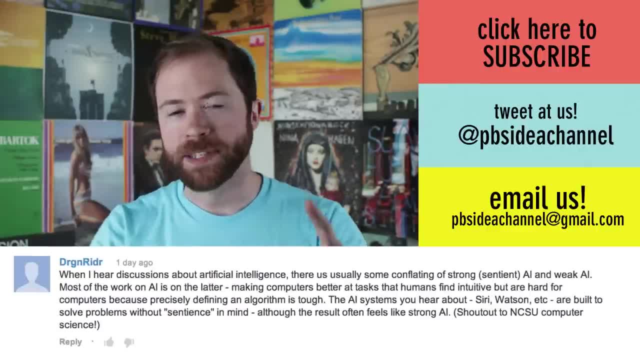 Which, yeah, maybe another episode for another day. Dragonrider points out that the thing that's missing from this conversation is a distinction between AI, which is essentially a consciousness, and AI, which is basically just reacting based on probabilistic models, which is a very fair criticism. 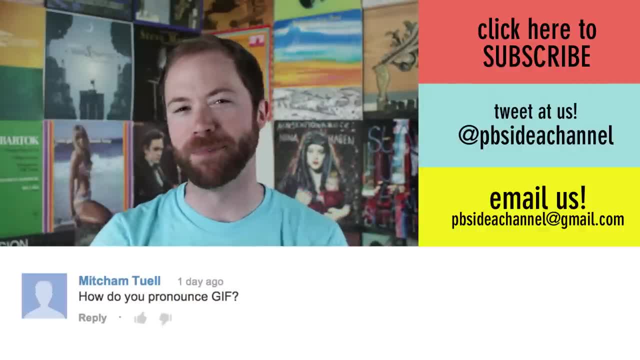 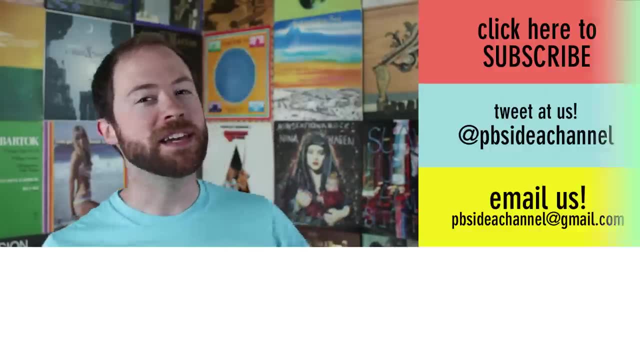 You know Mitchum Tool. I am so sick of this debate that from now on, I'm going to pronounce it zhaif. They're animated zhaifs. What's up now? This week's episode was brought to you by the awesome work of these naturally intelligent people. 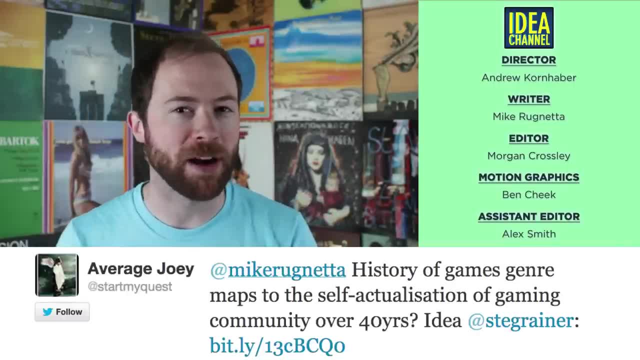 And the tweet of the week comes from Average Joey, who points us towards an article comparing the history of game development to Maslow's hierarchy of need. It's really good.